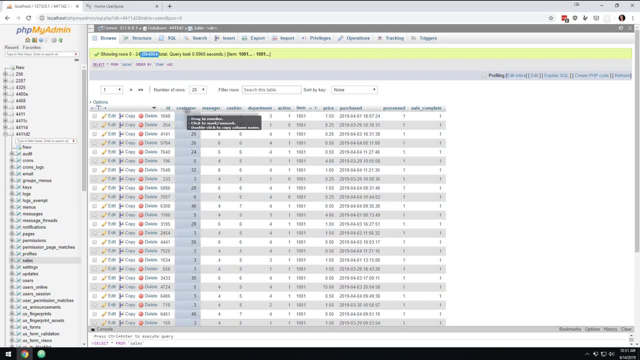 almost 875,000 rows in this thing And it's just a very simple- we'll call it a sales table- and it tells you the customer ID, the cashier ID, what department they bought the thing, from, what item, And this is the total. it's obviously not the price of the item. 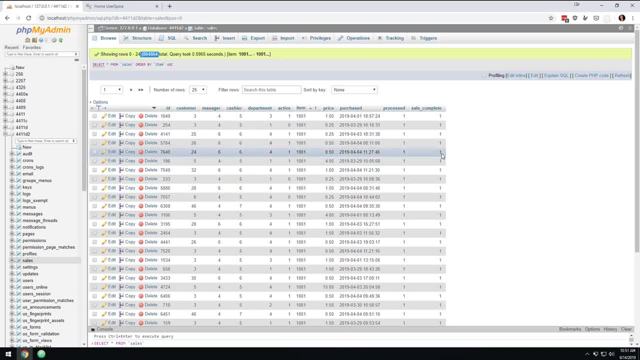 it's the total amount of that item they bought, what time, whether it's been complete, like nothing fancy in terms of data. There's just a lot of rows, And so let's say that what you would want to do. our challenge for the day is: we're going to go through and we're 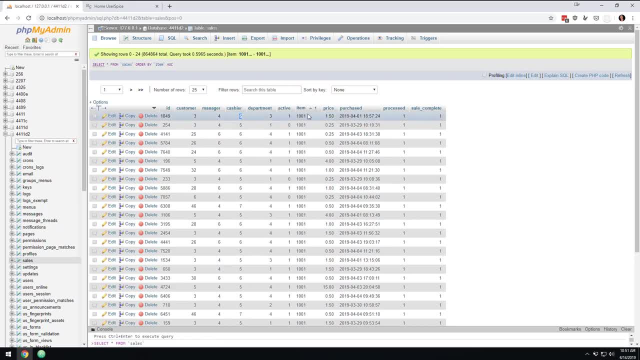 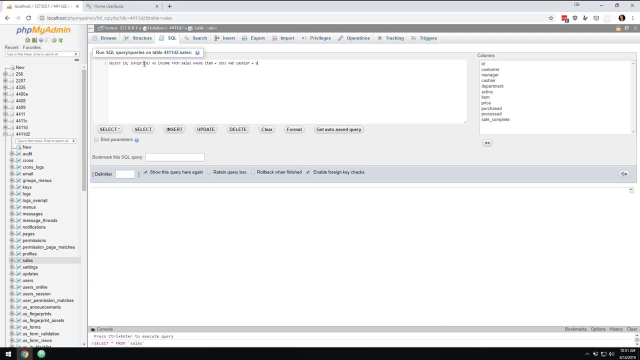 going to see how much cashier five sold of a particular item. And so if we were to come in here and just do a raw SQL query, I would say: you know, I want the ID of the item and I want to sum up all of the sales: that of item number 1,052, the cashier five sold. 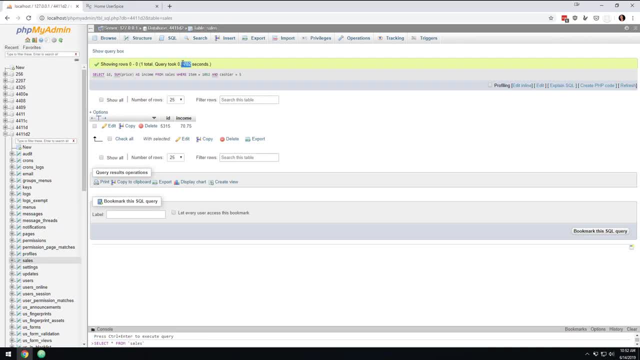 And so we're going to come in here and we're going to look and we're going to see it took about a third to a fourth of a second. sorry, a third to four tenths of a second. And so we're going to switch over to PHP and we're going to just look at this in just how it. 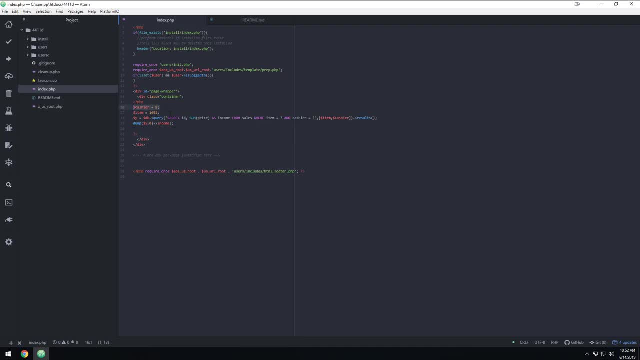 would look in your real world application. So we're going to say the cashier is five and then I've given it just this random number And we're going to do that same query And we're going to just dump the income. So if 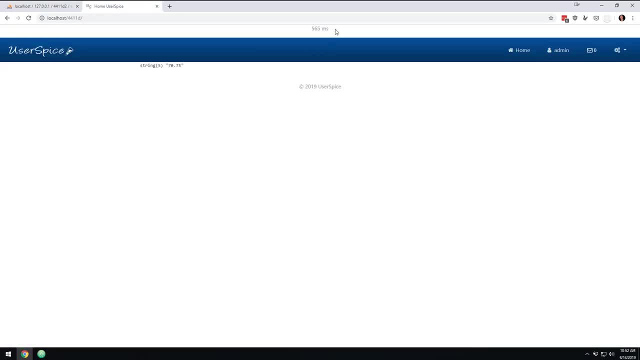 I were to come over here and refresh the page, you would see that the whole page loaded in 565 milliseconds, And so not terrible. UserSpice 5 is faster on this type of stuff. This is UserSpice 4.. You know so you think. well, what's the big deal? It took half a second. 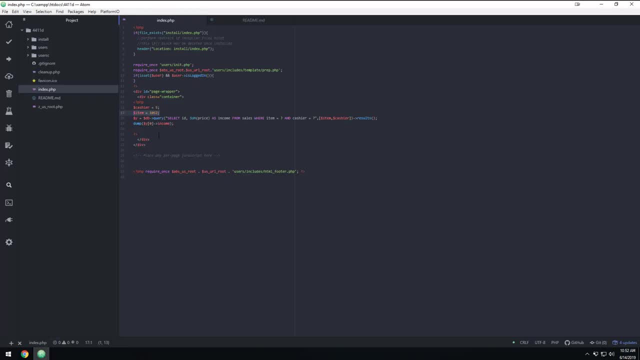 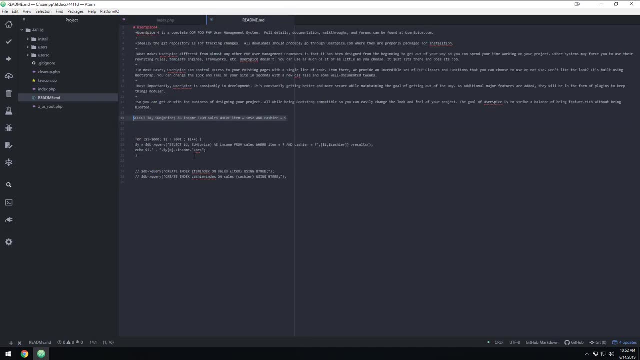 to load. Well, what if you want to do something like a chart? And what if you want to say: all right, we're going to forget this, but we want to show- I'm going to bring in another query here- We want to show what would happen if we went. 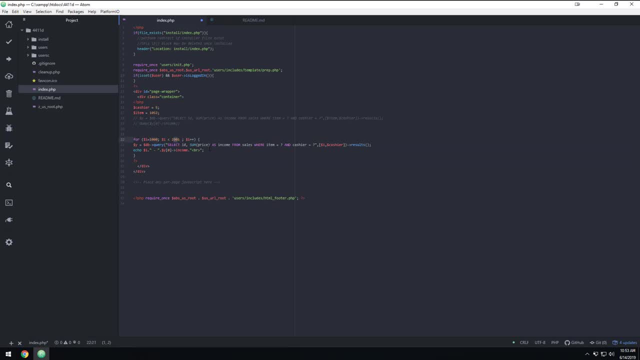 through every item, from item 1,000 to item 2,000, and we summed it up and we want to view how many they sold, or how much they sold. Well, for brevity's sake, I've already done that and I don't want to bring the. I don't want to make the computer do it again, because 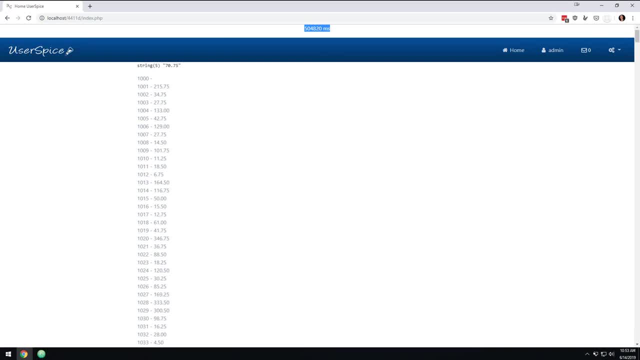 it took 500.. It took 504,000 milliseconds, which is 8.4 minutes, to run that query, to basically go through 1,000 items and find out how much of that did Cashier 5 sell And Cashier 5. 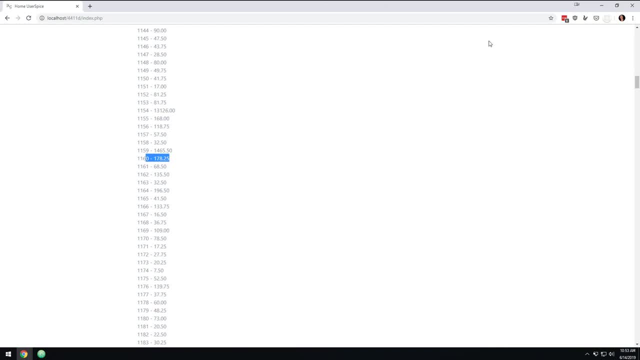 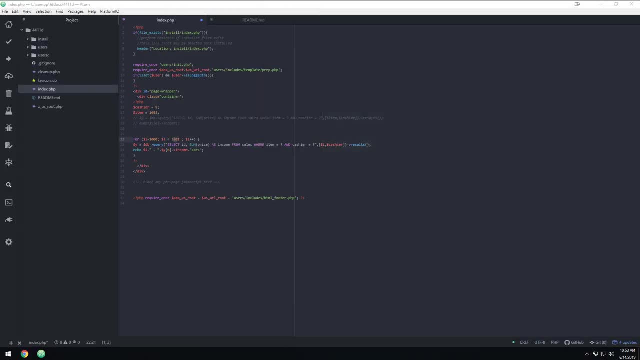 sold. you know 1,000 of this and you know 178 of that and all that That took almost eight, almost eight and a half minutes, which is just absolutely ridiculous. And if this was your application, you have thousands of items like you just can't have them run. 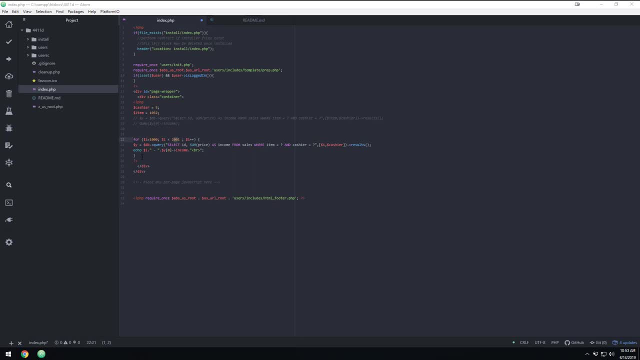 That long. And so the question is why? and it's because it has to go through the entire table and look for this item number, whether it's at the beginning or the end, And so we're going to use something called B-Tree And the best way I can explain it. there's a lot. 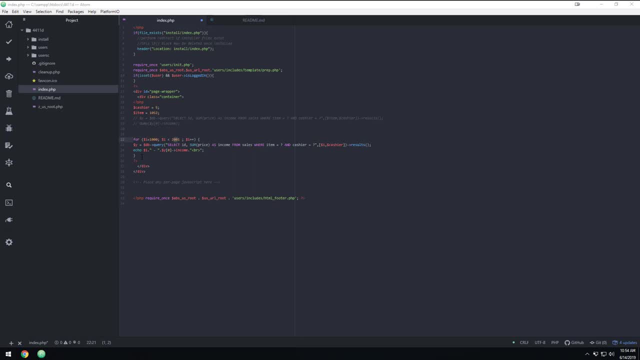 of really technical. you know there's a lot of really technical explanations on the internet. but let's just say you've got a room with a thousand people in it and they all have unique names and you're looking for Dan, And so basically, what would happen is you could. 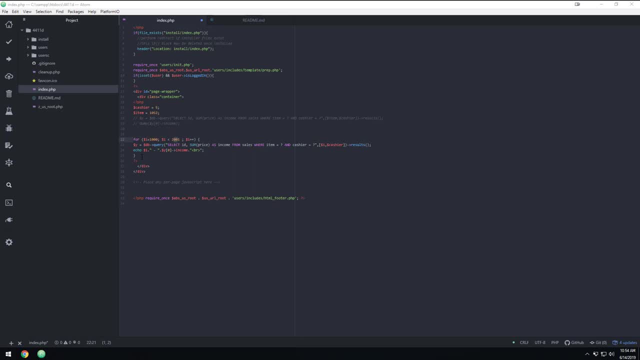 be each and every person and say: are you Dan, Are you Dan, Are you Dan? And you know, on average you're going to hit it about the 500th person. But what if you could have a list and say everybody on the left side of the room? their names begin with A through. 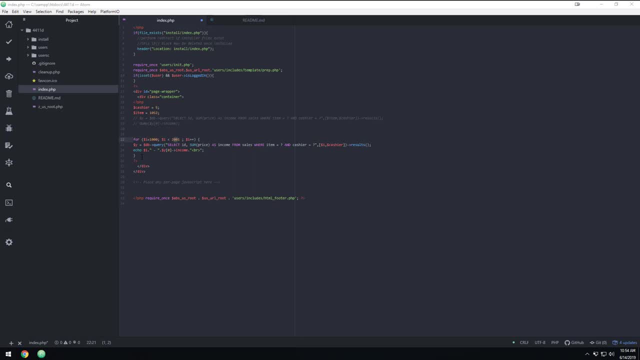 M and everybody on the right side of the room theirs begin with N through Z And then you say well, all right, And then in the first, in the front left quadrant, everybody is A through D. You know, all of a sudden you could start. you can kind of visualize the idea. 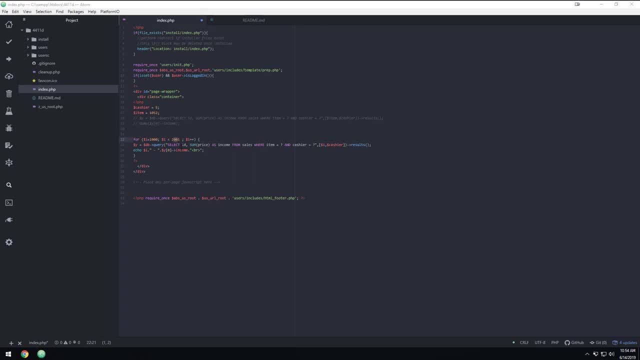 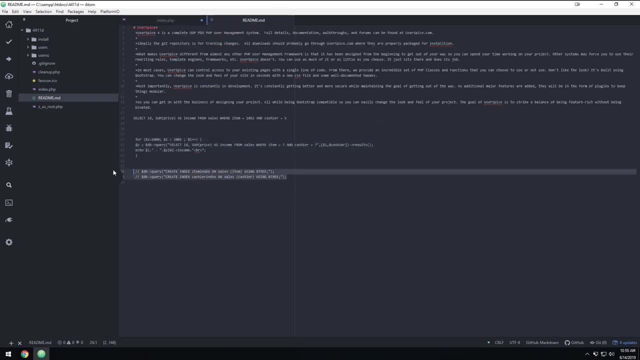 of narrowing down your search query and not having to look through as much of the database as before. So what we're going to do, I'm going to do something. I'm going to drag these queries in real quick, cause I'm going to show you how they work, And we're going to 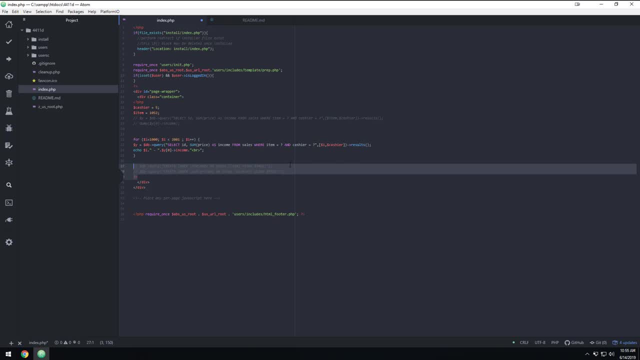 do this in PHP. We could just as easily run this in PHP, my admin, but I'm going to comment these in for a second and I'm going to comment everything else out. So what I have here is a very simple database query: create index And then what you're. 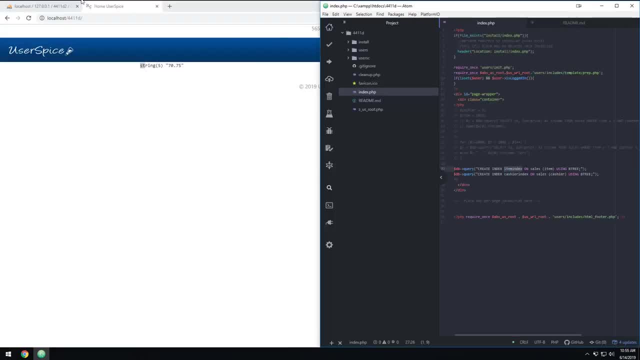 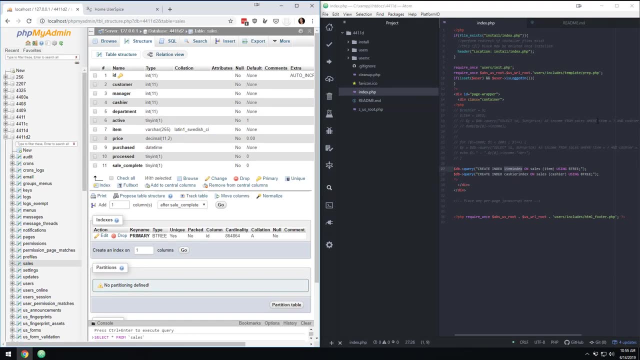 going to do is you're going to give it a unique index. Now, let me, I'm going to snap this over here so we can look at the database. So what you can see if you look here, we are searching where item equals something and cashier equals something, And so, basically, 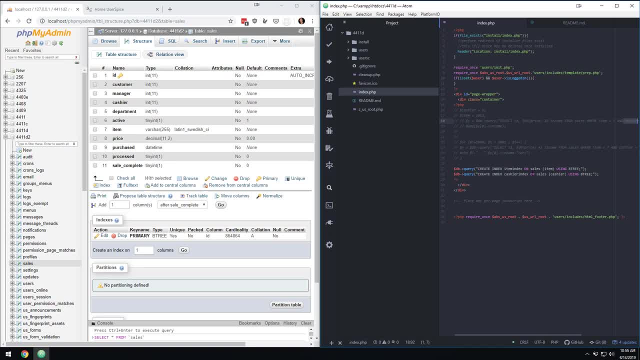 what we want to do is we want to say, Hey, item and cashier are important And they're things that we're going to search the database by, So we need to be able to find these quickly. So what we're going to say is: we're going to create an index and we're going to give 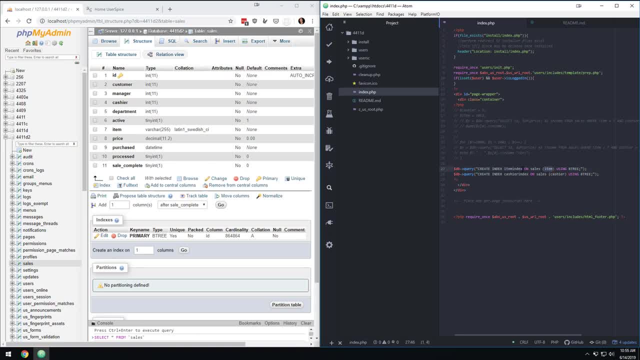 it a unique name And we're going to say, Hey, I'm going to create a unique index And we're going to create one on item, And so I like to call it item index to make it really simple. And then we're just going to say: using B-tree and same thing: cashier index on cashier using. 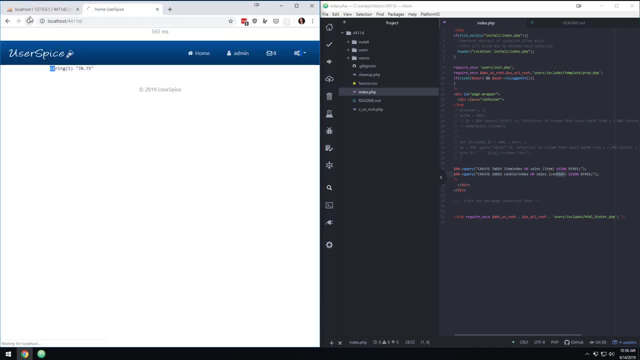 B-tree. So I'm going to save this and I'm going to refresh the page. It's not going to do anything. Let's see. Let's make sure that, actually refreshed, Hit enter. What's going on there? Okay, There we go. So we refresh the page so I can comment this out. We don't. 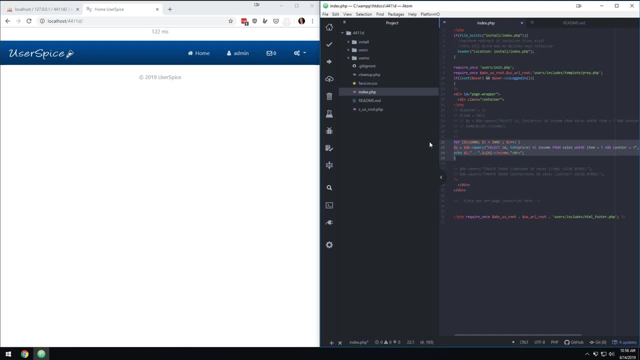 need it anymore. And then we can come in here and do this Same thing. we're going to say: I want to see everything from item 1000 to item 2001.. Add them up and echo out the prices, just like we did here. The only difference is that it's 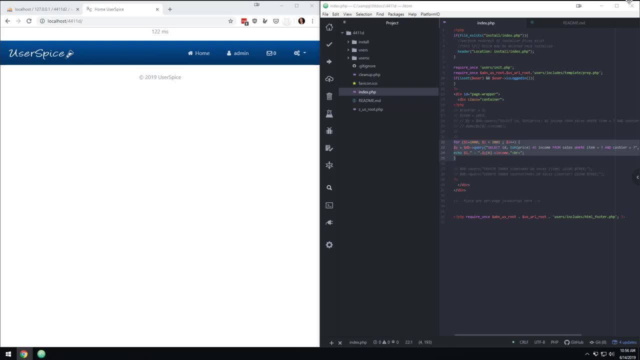 not going to take 500,000 milliseconds. So we're going to save, We're saved and we're going to come in here. I'm going to hit enter, I'm going to reload the page and it's not going to be instantaneous. I don't think. so. Yeah, there we go. It's not, It's funny. So 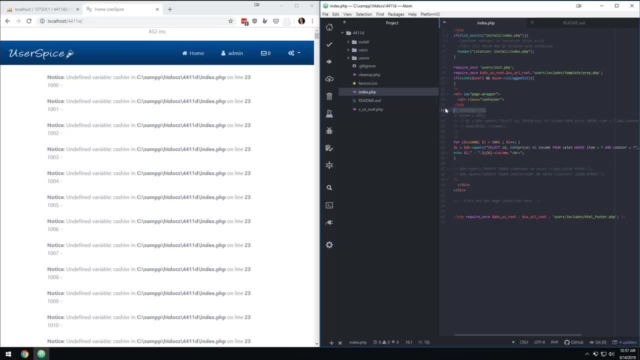 if you're following along, I'm sure you saw what I did. I'm going to hit enter and I'm sure you saw what I just did. I had cashier commented out, So I'm going to comment that back in and I'm going to hit enter again And we're going to make sure the page is actually. 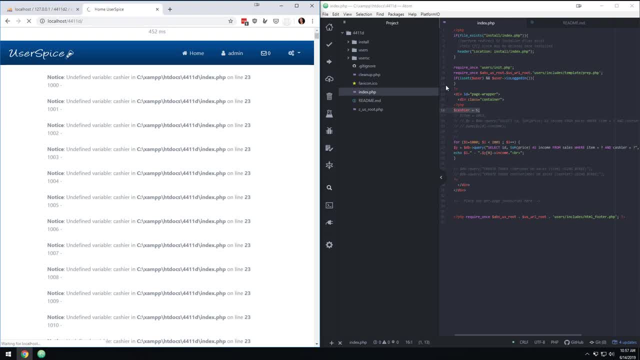 loading this time And you'll see that it should take eight to 12 seconds, something like that, Maybe a little bit more, to go through and do all of that. calculations. All right, Yeah, 11 seconds, So not instantaneous, And there are some other things you could do to.